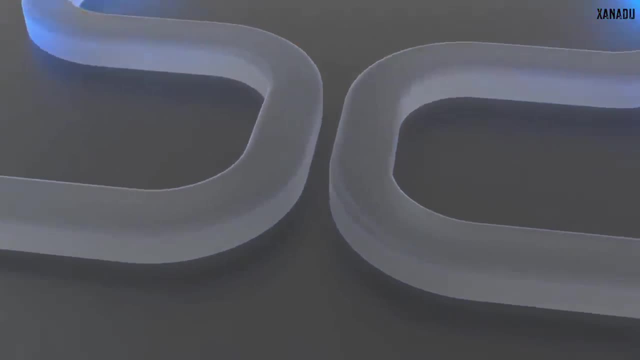 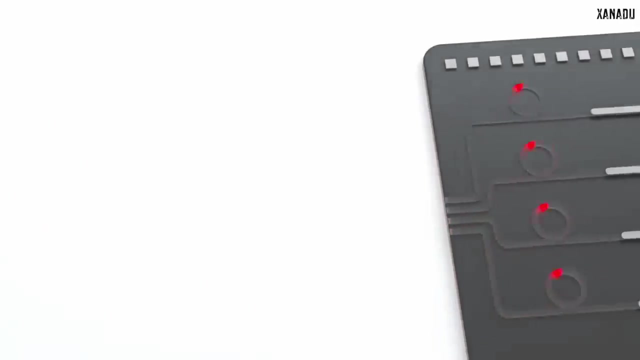 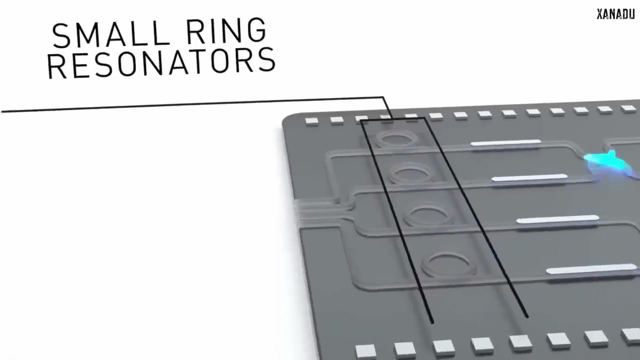 can also exist in a superposition of these two states, So it is zero and one at the same time. These photons are usually generated by a bulky external laser. Then to perform operations on these photons, we use mirrors and phase shifters to create entanglement between photons And this. 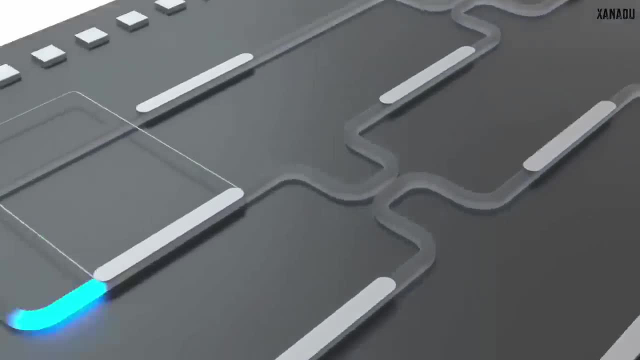 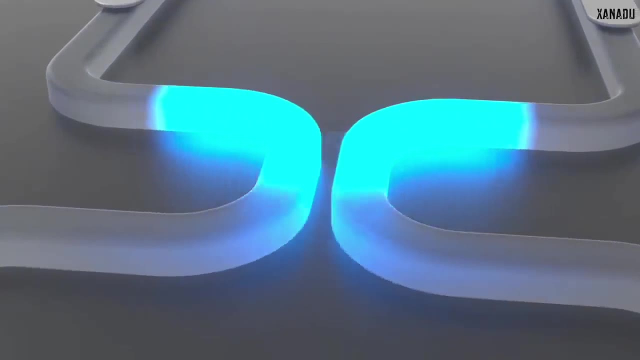 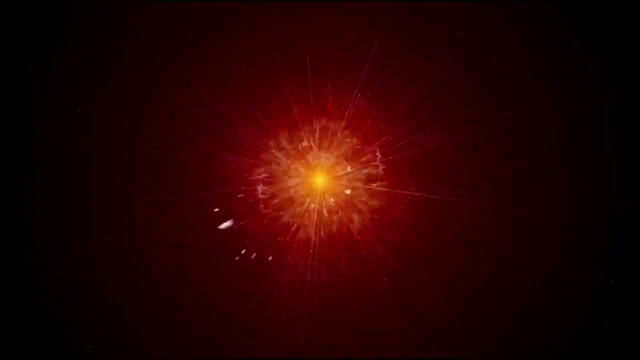 entanglement is the key to performing quantum algorithms. When two photons are entangled, they are connected And they affect each other, even if they are light years apart, And it's mind-blowing just to think of this, you know. Think of Big Bang, when all those particles were so densely packed together. 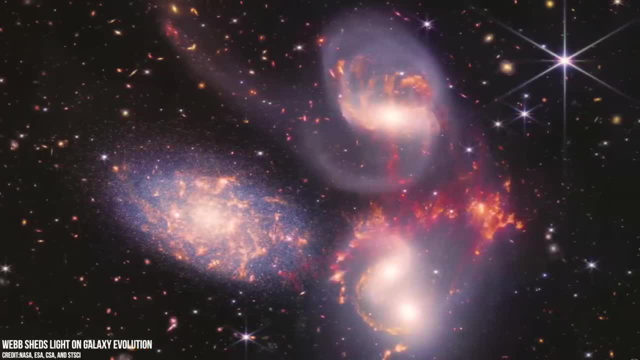 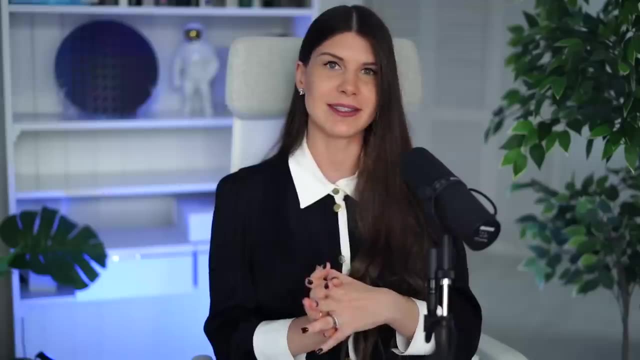 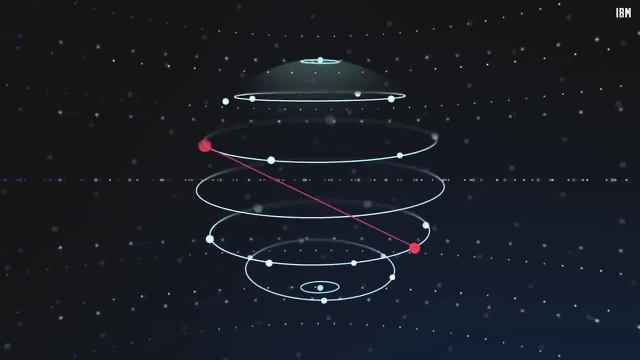 and now they are spread all over the universe, still entangled, And some of these particles are a part of us. I like to think of this. Photonic quantum computers have many advantages over those based on electrons. First of all, photons are much more immune to the environment. Photons do not. 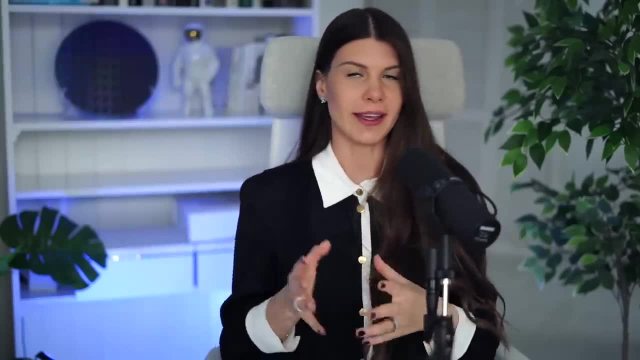 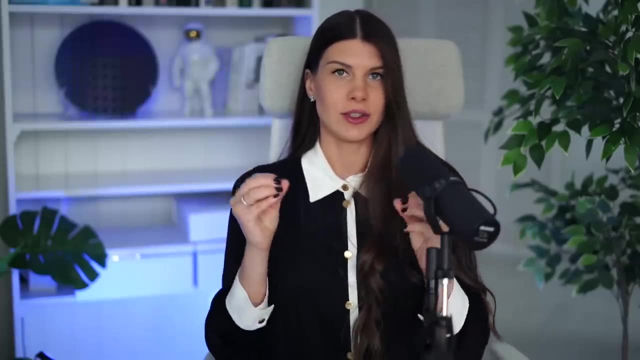 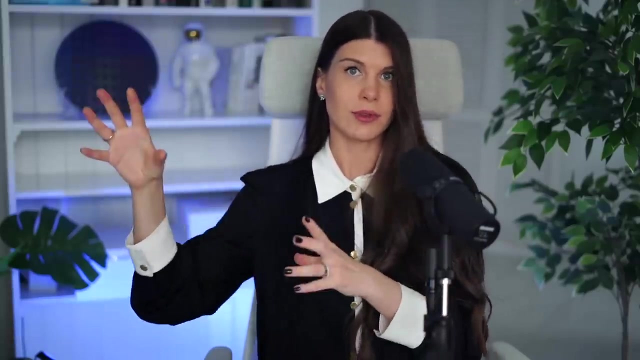 interact that much with the environment. That's the reason why they can operate at room temperature without any cooling. And also this is a big plus in terms of scaling, Because it makes it much more easier to scale photonic quantum computers to larger number of qubits And also building a more 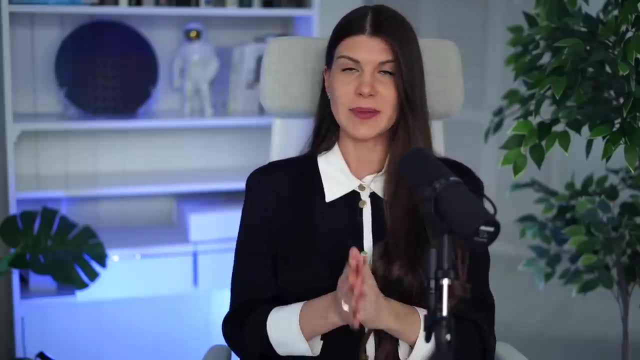 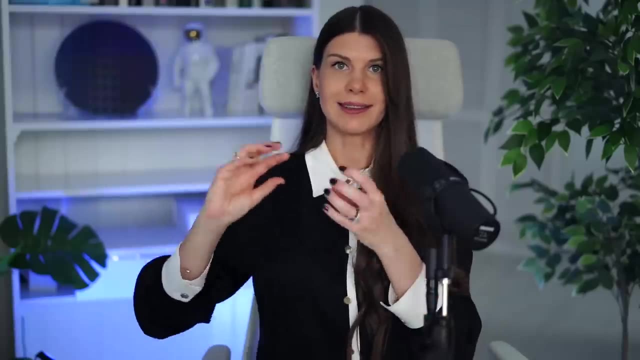 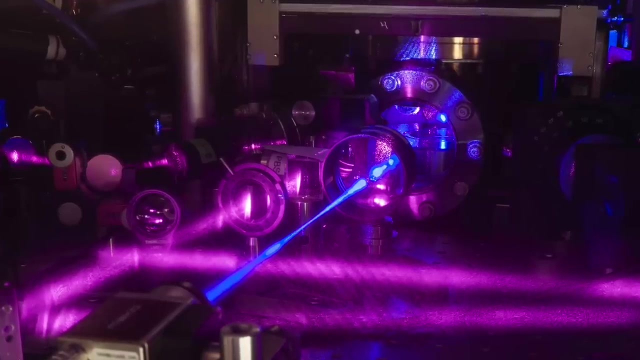 portable quantum computer Sounds cool, right, But here is the problem: In order to make photonic quantum computers to work, we need to generate entangled pairs of photons. Till today, to generate this light and its quantum states, we used bulky optical equipment. 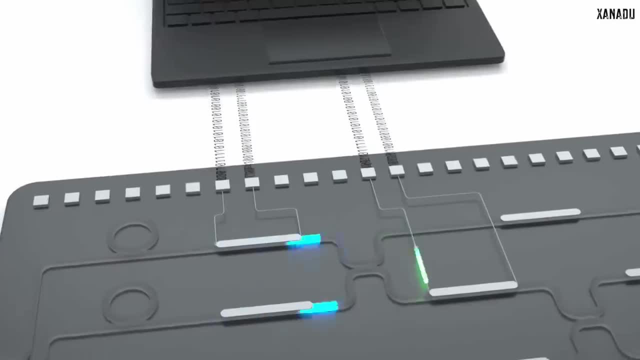 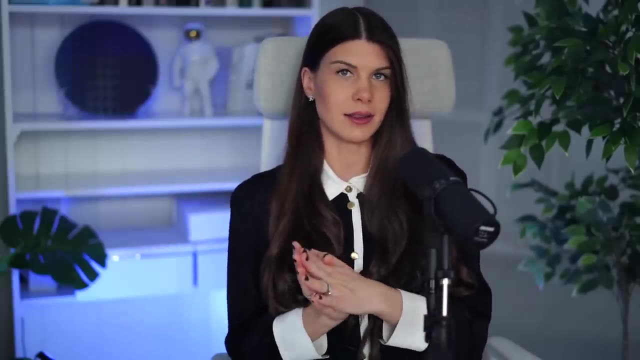 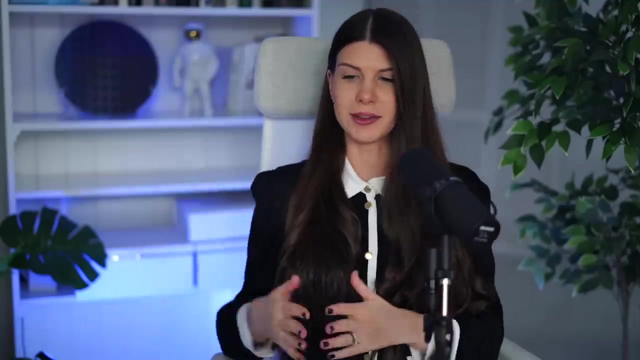 For example, huge lasers like this and many large beam splitters. But we know that everything what is bulky like a classical qubit, it's very hard to scale And eventually we want a device which fits in our pocket or on the table right. 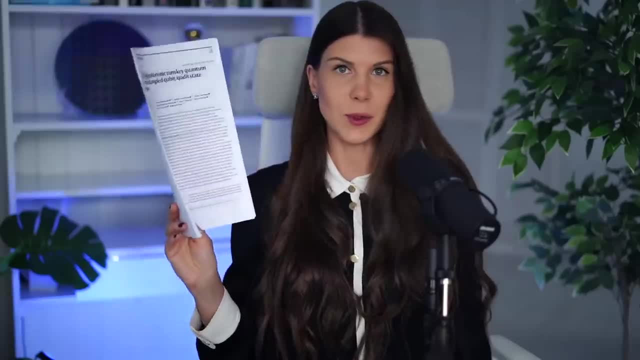 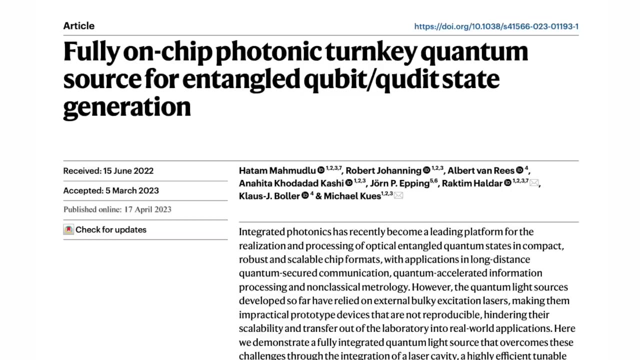 Not a computer which occupies the entire lab, And in this new paper they solved this problem. This is the new paper which came out just few days ago. Here they've built the first photonic chip for quantum computing that integrates all the required components. 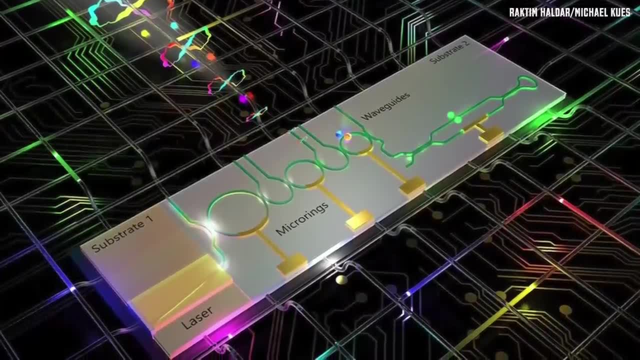 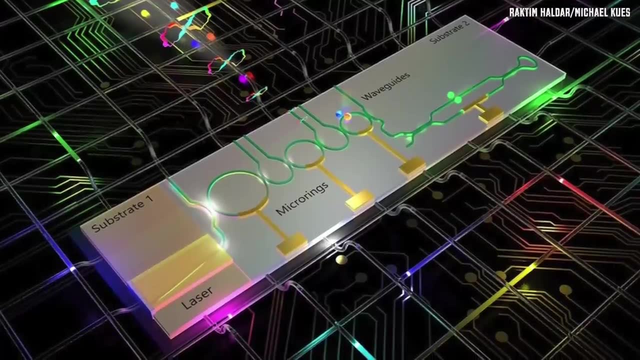 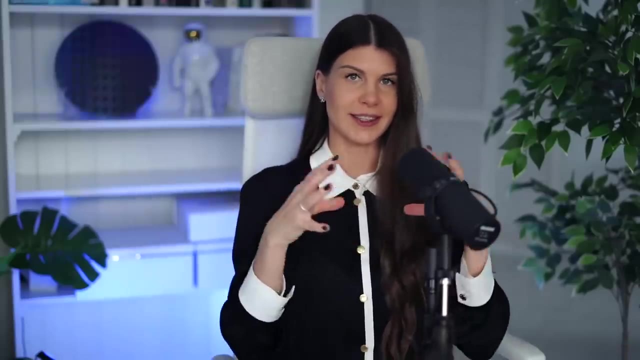 All the required functionality into a tiny chip, 1 to 1 cm square. Dutch researchers were able to integrate all the complicated optics and filters together on a single chip. What is truly fascinating is that they were able to shrink the size of the laser. 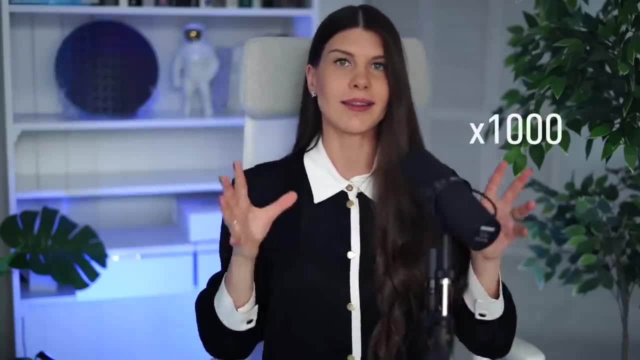 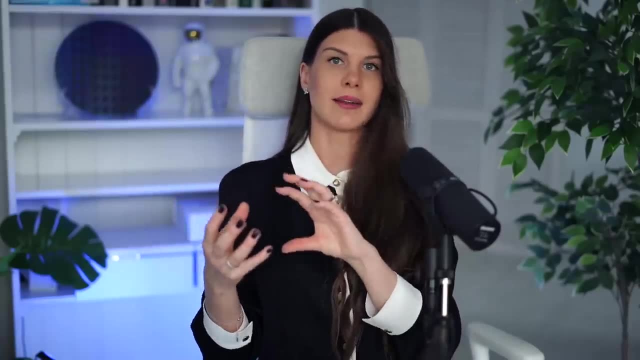 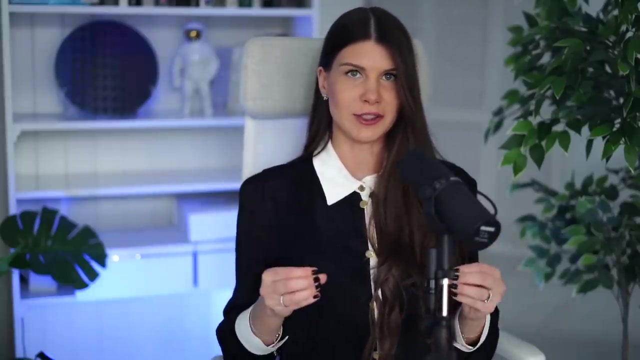 so the size of the light source by 1000 times. Oh wow, This new chip can both generate photons on a chip and entangle them without all of this bulky equipment. So basically they solved the problem of integration. This new chip combines two emerging technologies. 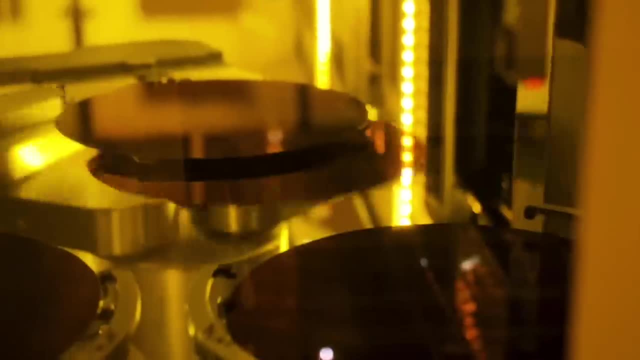 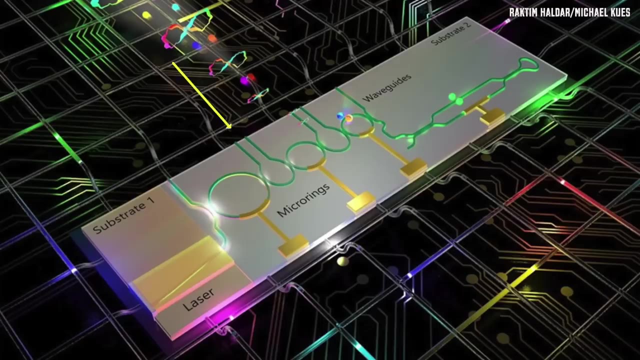 A laser made of indium phosphide and a filter made of silicon nitride. The first section generates the light And then they filter out the noise from the light, so it doesn't interfere with the quantum states. Then two photons are abolished to generate an entangled pair of photons. 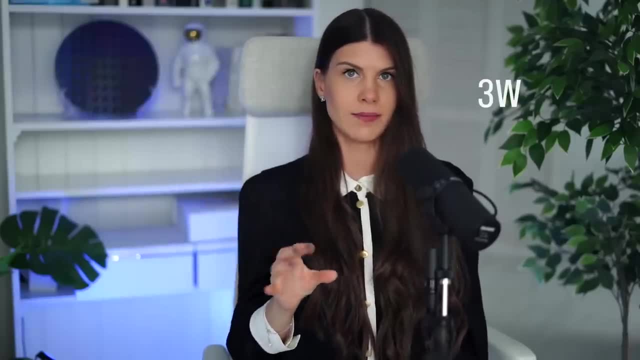 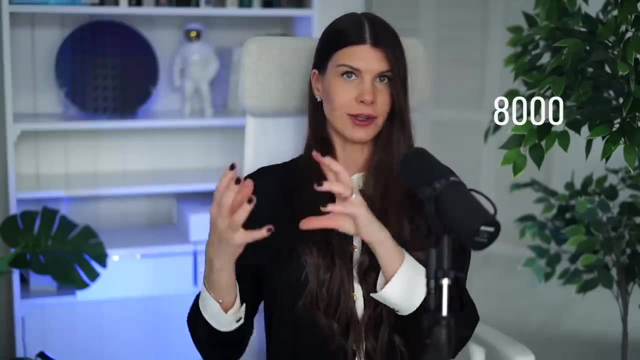 This chip draws about 3 watts of power, which is honestly quite a lot, And it's able to generate 8000 pairs of entangled photons per second. This is such an amazing progress. Let me know what you think in the comments. 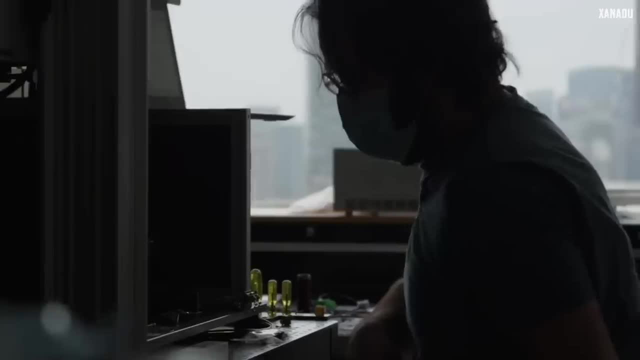 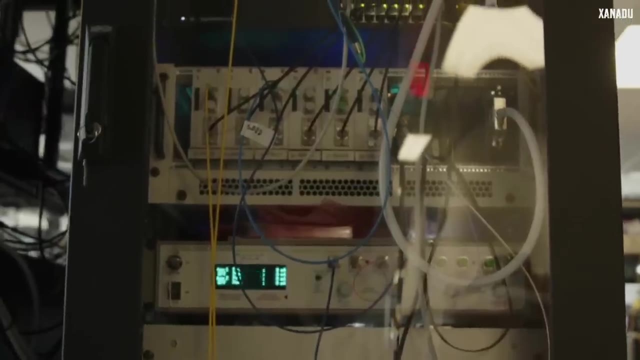 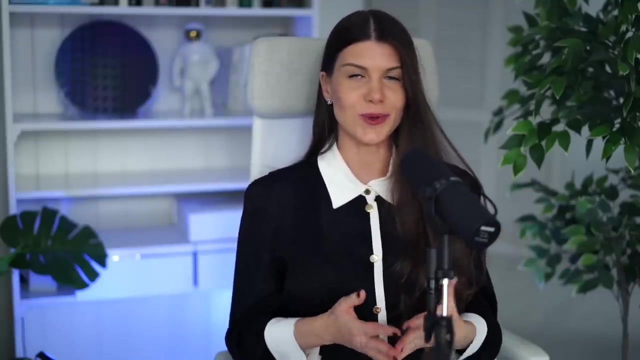 What makes this technology so appealing, that photonic quantum computing has many advantages over other types of quantum computing. It is definitely better scalable and also it's more robust against noise. And this is already covering the main challenges which we are facing with classical quantum bits. Also, they are easily integratable with modern telecommunication systems through an optical fiber. This means we can easily scale photonic quantum computers, build it in a cloud and even build the quantum internet to connect them. That internet, theoretically, will be much more secure. 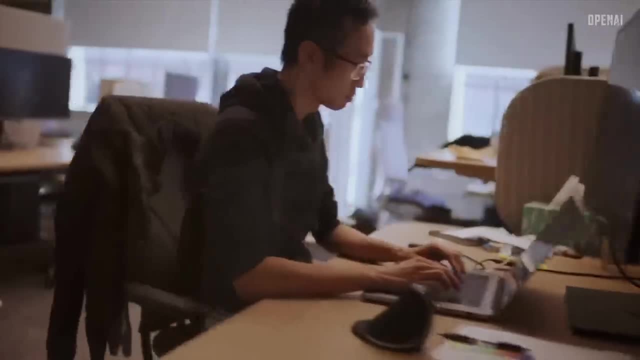 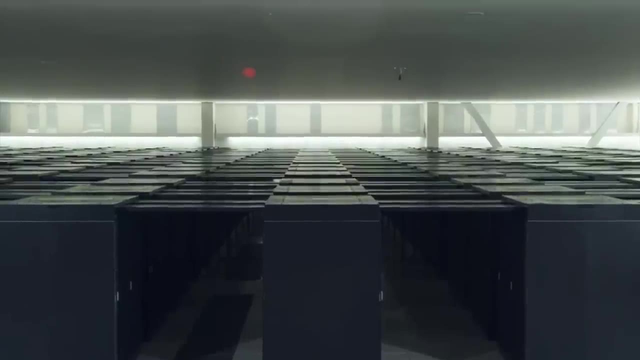 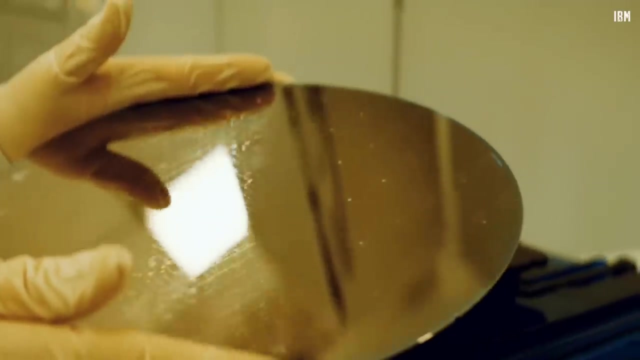 and much more powerful than the modern internet. In general, photonics is already widely used in many other applications: in telecommunications, in photonic computing and in sensors. This means there is already a mature infrastructure for manufacturing of these devices, And all of this makes it easier. 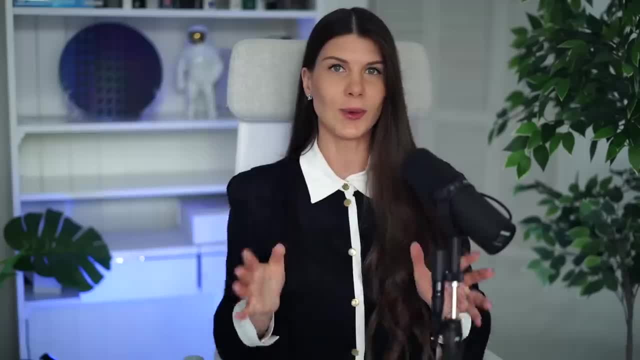 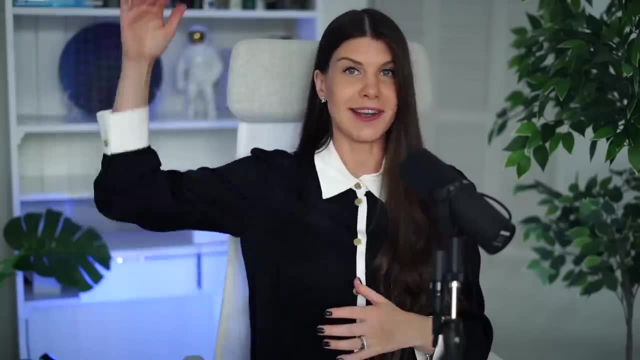 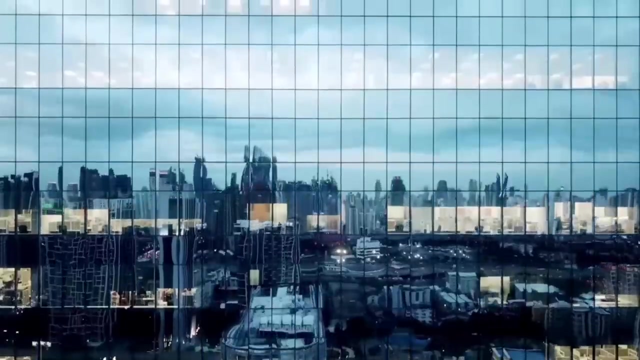 to develop and scale this technology. Why is this research important? Because photonic quantum computing has the potential to generate exponential speeds up in science And eventually the goal is to make this world a better place. For example, we will be able to simulate: